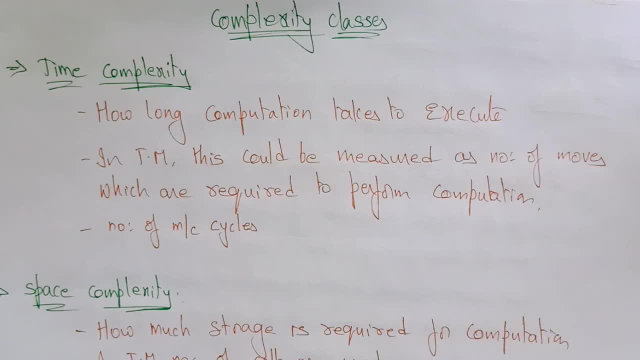 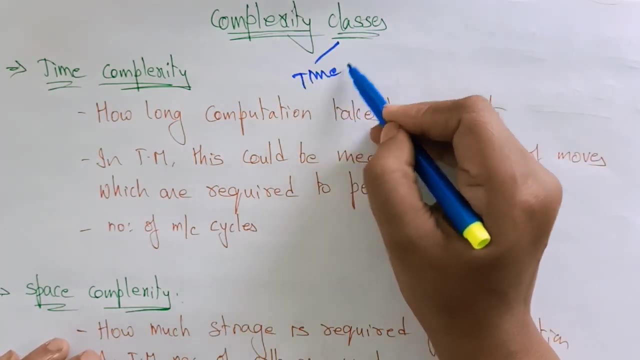 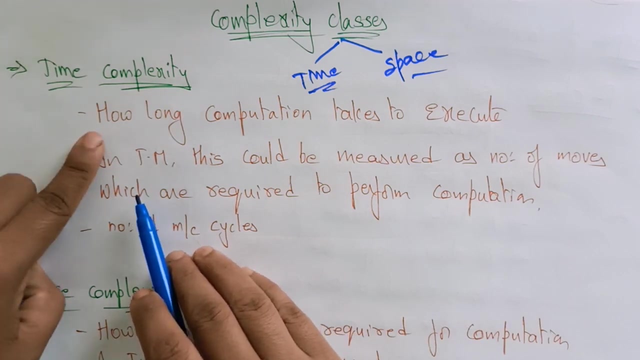 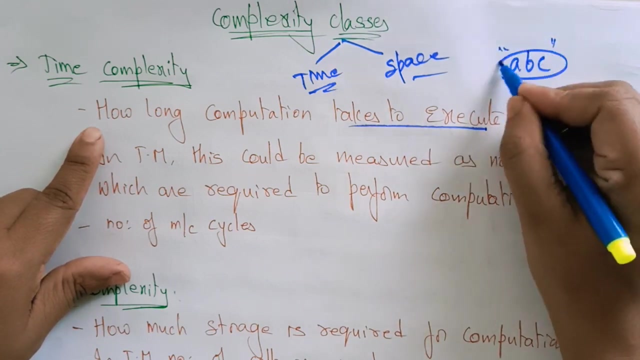 Hi students, welcome back. Coming to the next topic in the subject theory of computations is the complexity classes. So the complexity classes is of two types: means we are based on time complexity or on the space complexity. So what is the time complexity? Time complexity means how long the computation takes to execute. So, whatever, we are taking a string, Okay, So how long that the machine is computing. this string means how long the computation takes to execute. 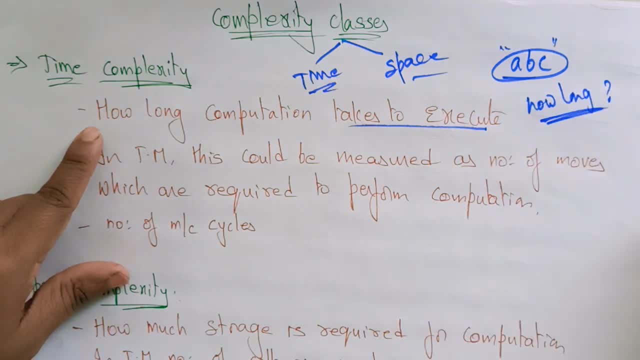 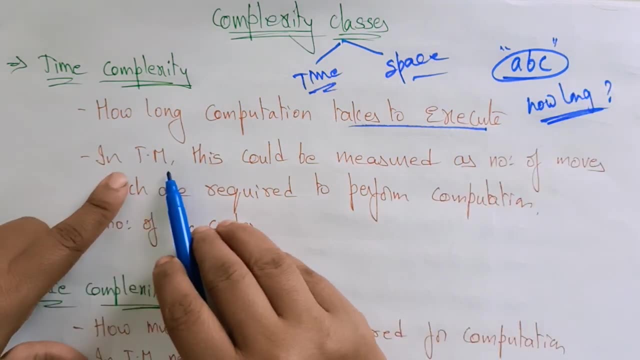 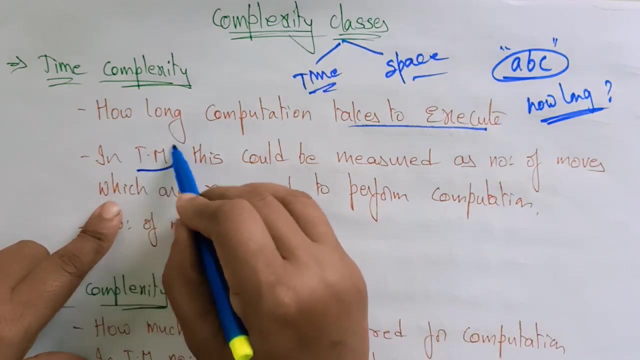 that is a time, how long there is a term time complexity- so how long the computation takes to execute is determines the time complexity. in a Turing machine this could be measured as number of moves which are required to perform a computation. so in the Turing machine, how you decide the time, 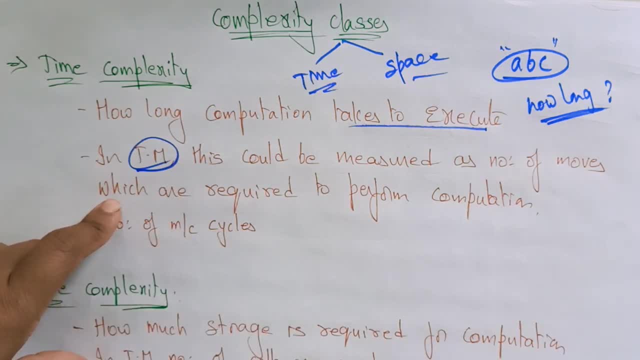 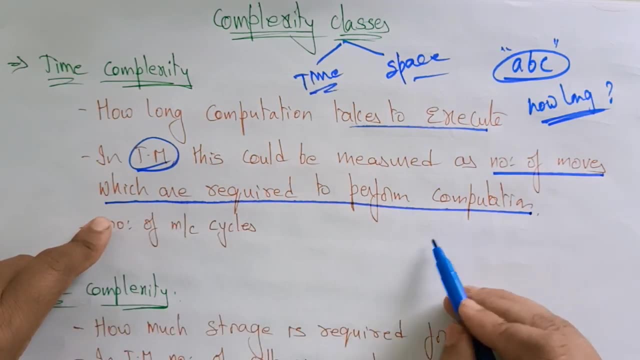 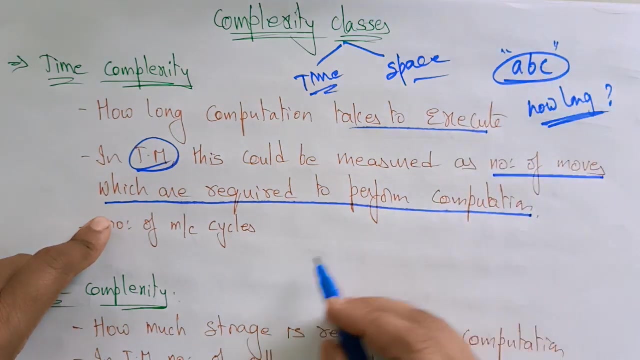 complexity, how you find out the time complexity. so, that is, it is completely based on number of moves which are required to perform the computation. suppose I want to compute this. sorry, this alphabet, this is this ember. okay, so this is an input. I want to compute in the Turing machine. so how much so? how? 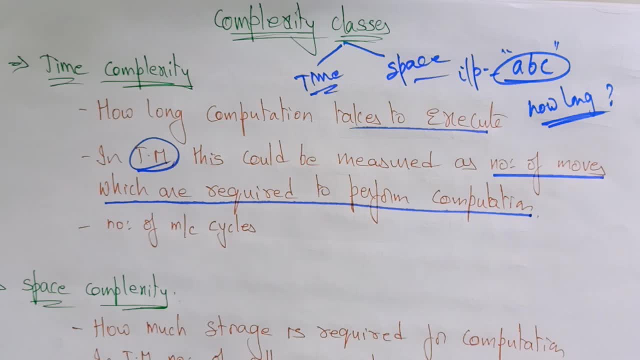 much. this could be measured as number of moves which are required to perform computation. so that is a number of machine cycles. okay, it's completely on number of moves which are required to perform computation. so that is a number of machine cycles. okay, it's completely on number. 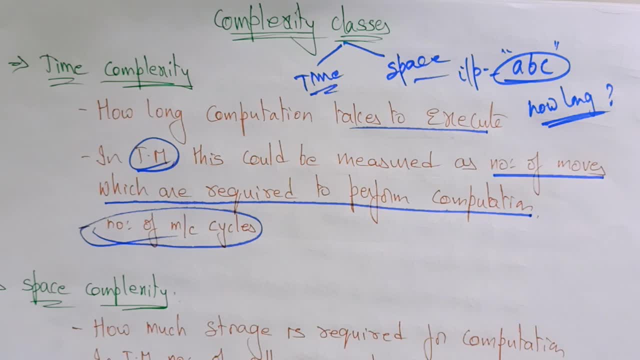 of machine cycle means which measure number of moves which are required to perform a computation. now put some Q naught okay, from taking the input and the next state and right or left, so how many number of moves it is taking to access the string. so that is represents, on the time, complexity. then what about? 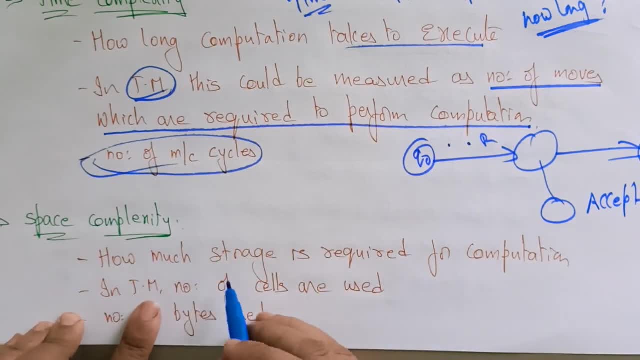 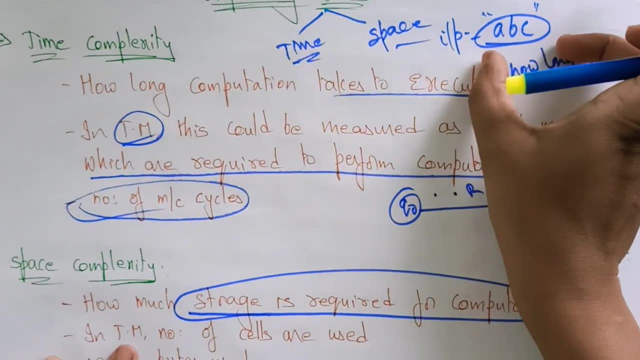 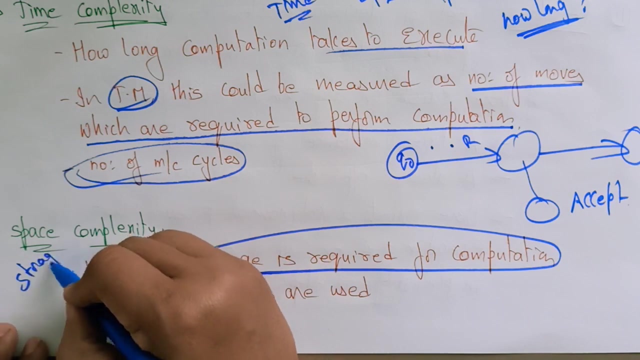 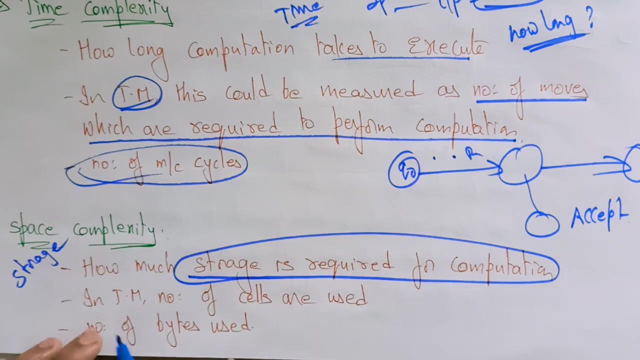 the space complexity. space complexity means how much storage is required for computation. so to solve its input, to solve that problem, how much space is required for computation? that is a space. space is storage. time is how much time it takes to complete that equations. okay, so the space complexity is how much storage is required for computation in Turing. 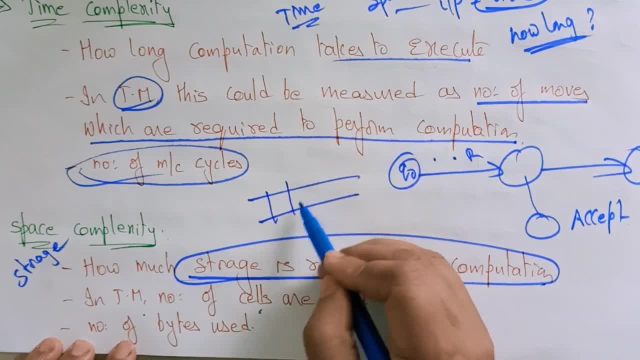 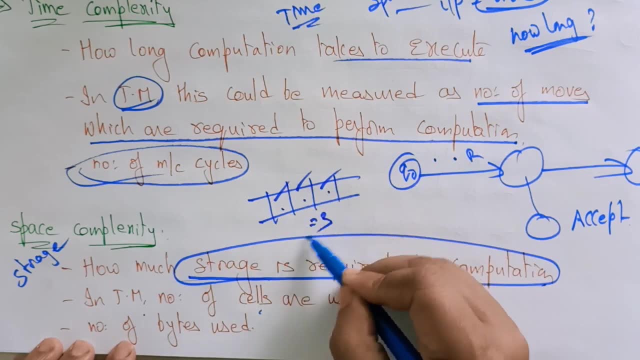 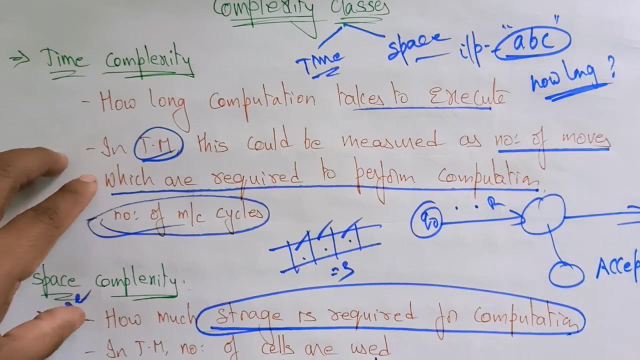 machine number of cells are used. so here we are using in the tape how many cells that are used. that depends upon the space complexity. here we are using three cells. okay, the space complex complexity is three, okay, so the number of bytes we are using. there is a main concept of time. 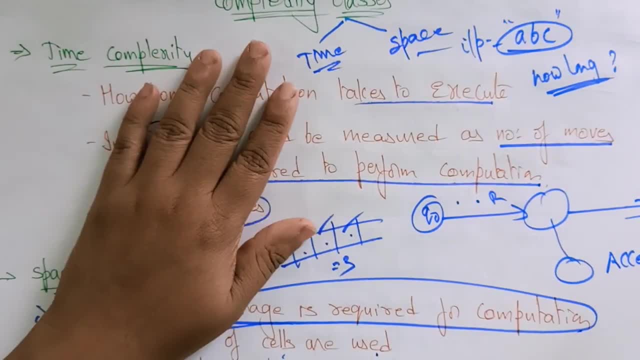 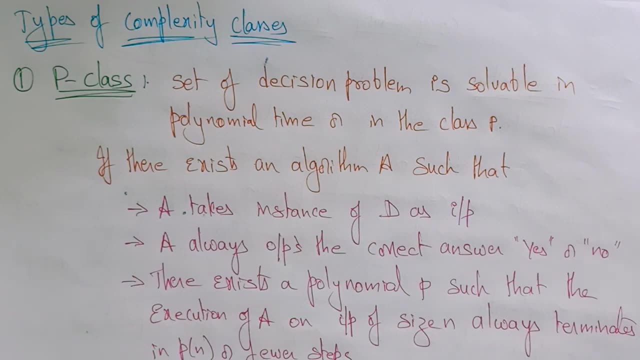 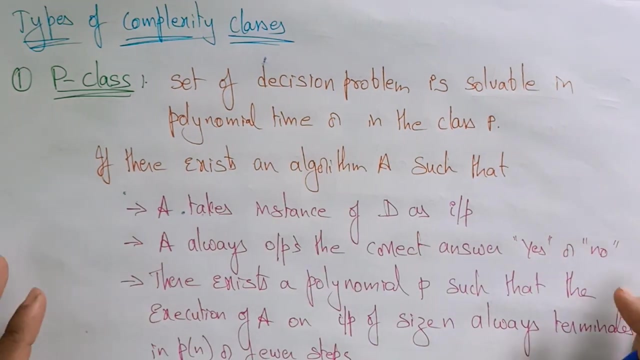 complexity and space concept complexity. now, coming to this complexity classes, there are different types of complexity classes: P class, n class, NP class- okay, completeness of NP, like that. so different types of classes are there, so I want to explain you some of the classes we are regarding this complexity. 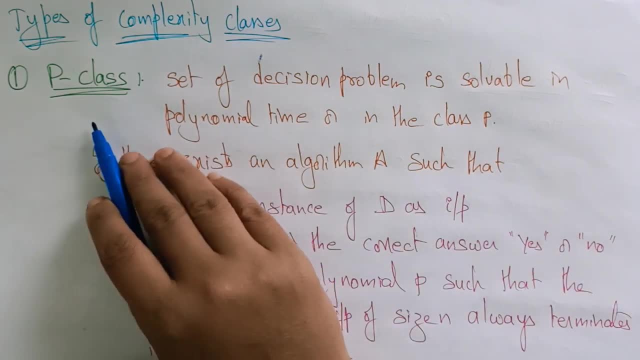 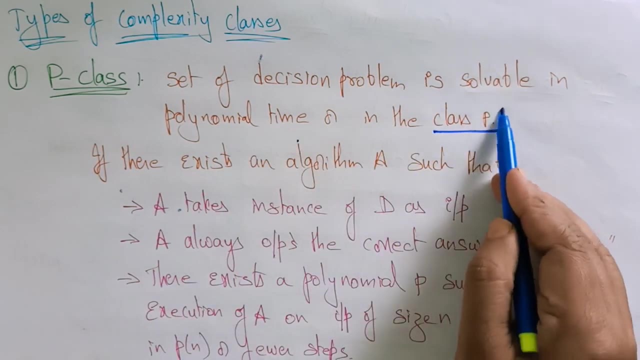 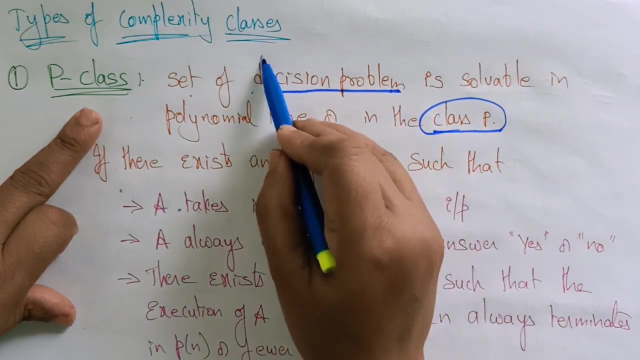 classes. the first one is a P class. so what is this P class? the second one is a set of decision problems is solvable in polynomial time or in the class P. that is a P class. the P class definition is here. I'm set of decision problems set. 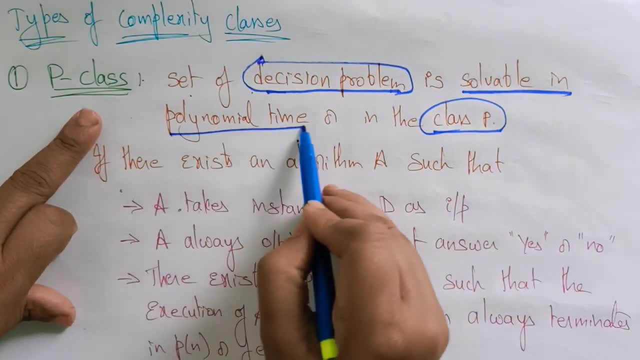 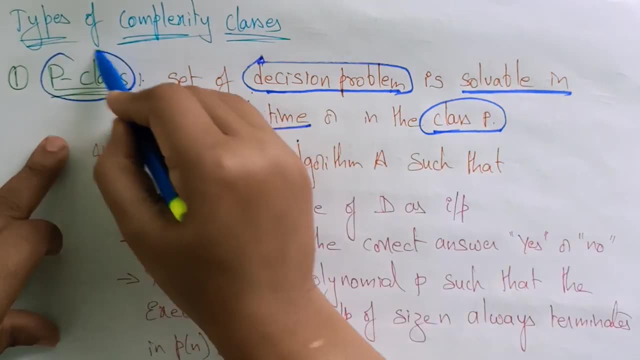 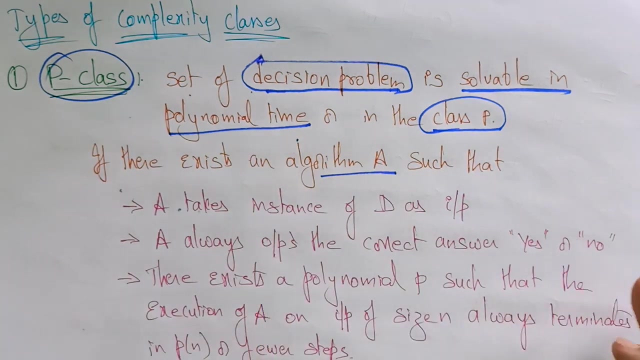 of decision problems that are solvable in a polynomial time. in a polynomial, in a particular polynomial time, I am solving the set of decision problems that you represents, the P class. so if there exists an algorithm a, let us assume that if there exists an algorithm day a, such that it takes instance of D, 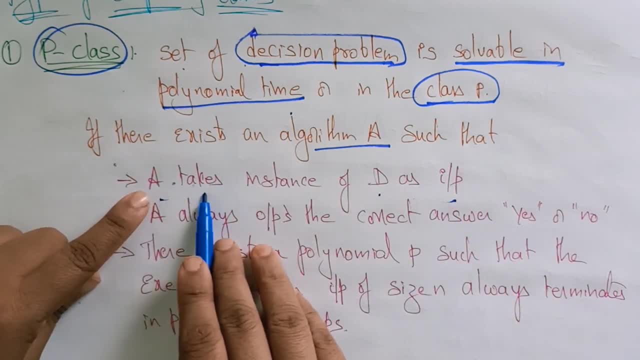 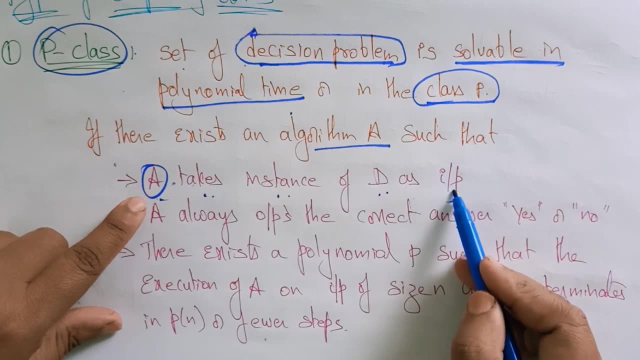 as input. okay, it takes instance algorithm a. okay, a is an algorithm, so a takes instance of D as input. now, a always outputs the correct answer. either s or no means, because this is a decision problem, you have to take it as s or no. there exists a polynomial P, such that the 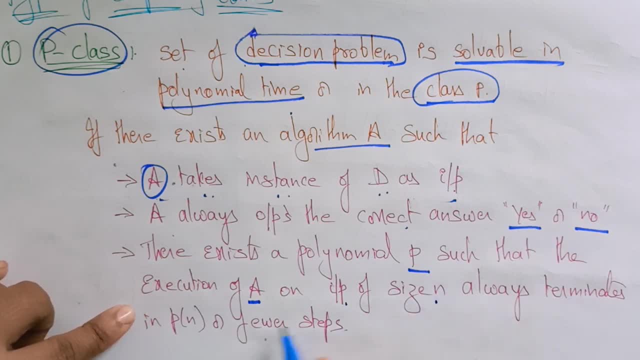 Execution of A on input of size n, always terminate on P of n, Because there exists a polynomial P, So such that the execution of algorithm on input- I am taking the size n, the space complexity is the size n- Always terminate it at the P of n or at fewer steps. 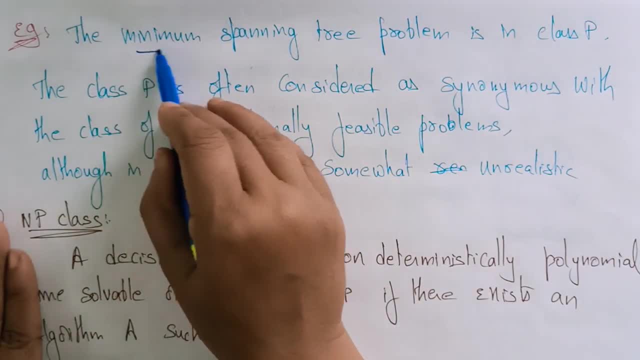 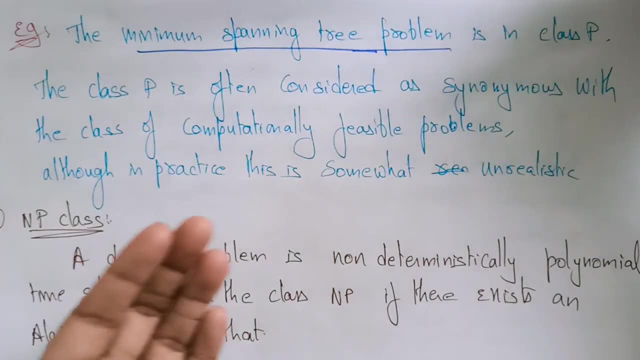 So the example for this P class is the minimum spanning tree. Okay, the minimum spanning tree problem is in class P. If you want to know about this minimum spanning tree, just see my previous videos in other subject. Okay, in the dark. 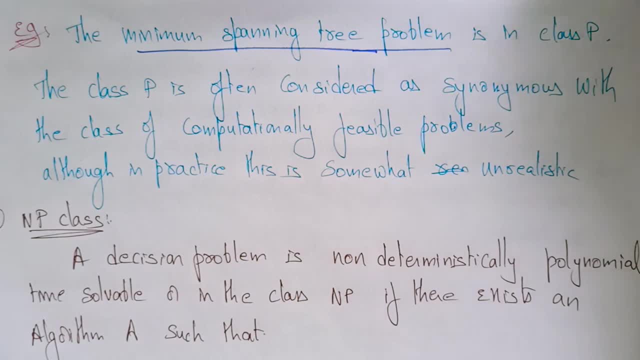 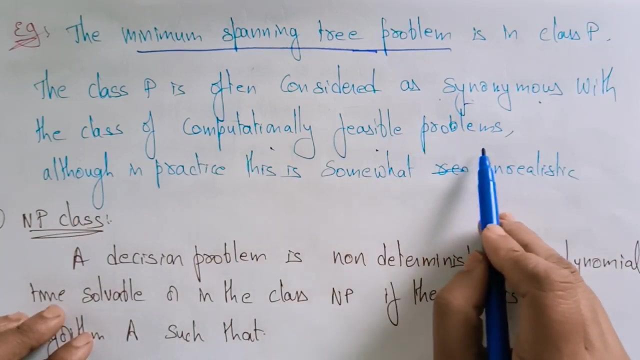 So there I explained the minimum spanning tree. So the minimum spanning tree is in this class P. How can I say this is in class P? Because there the set of decision problems is solvable in a particular polynomial time. So the class P is often considered as a synonymous with a class of computational feasible problems. 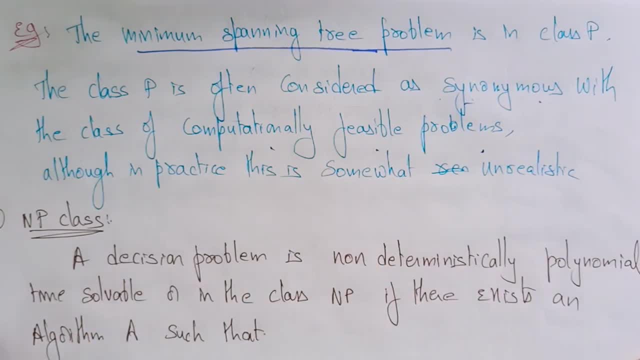 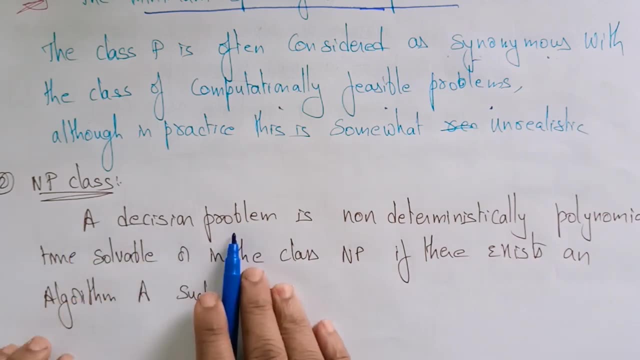 Although in practice this is somewhat unrealistic. Now coming to the next problem, Coming to NP class. What is this NP class? So NP class is non-deterministic. A decision problem is non-deterministically polynomial time solvable. 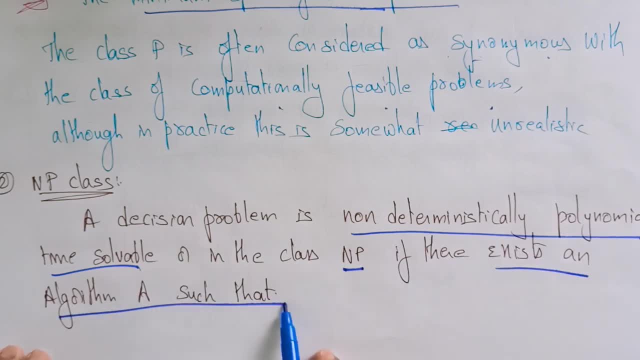 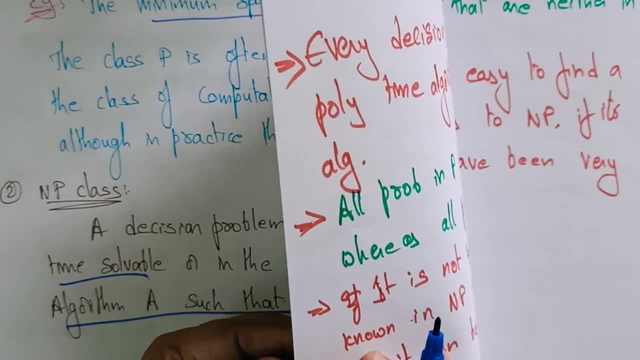 Or in the class NP, if there exists an algorithm A such that Means the NP class means it is a non-deterministically polynomial time solvable. Or you can take this algorithm: So here in this algorithm there exists a polynomial P. 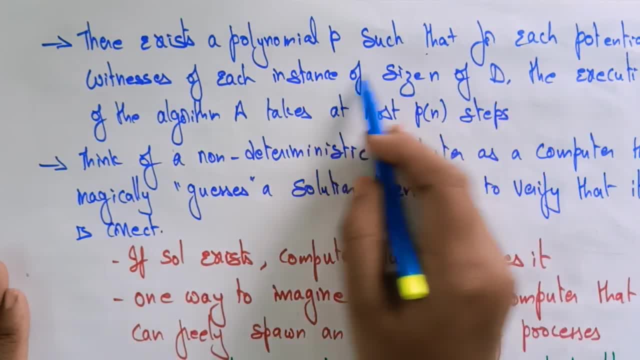 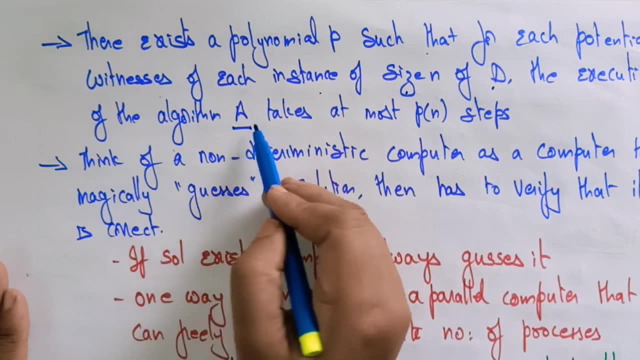 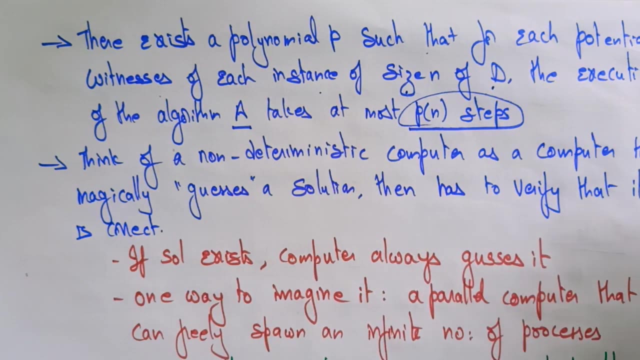 There exists a polynomial P, Such that for each potential witness of each instance of size N of D, There exists an algorithm A that takes in P of N steps. So, just like P class, it is just taking the each instance Algorithm A takes at most, not always terminates. 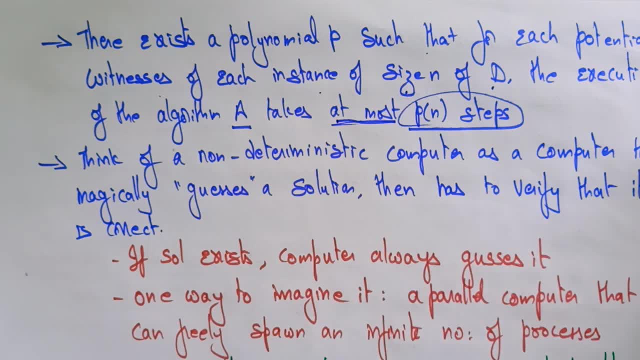 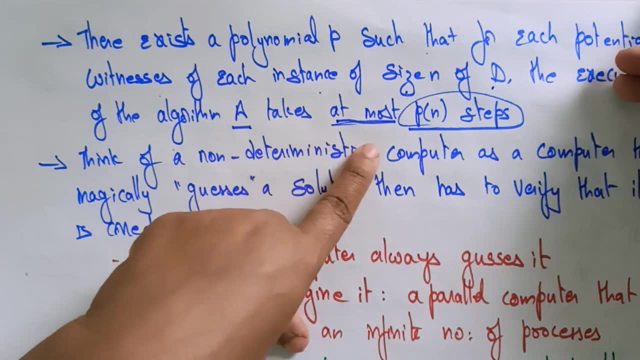 It takes at most P of N steps. So there in P class the size of N always terminates in P of N. But here the execution of algorithm A takes at most P of N steps. So think of a non-deterministic computer as a computer. 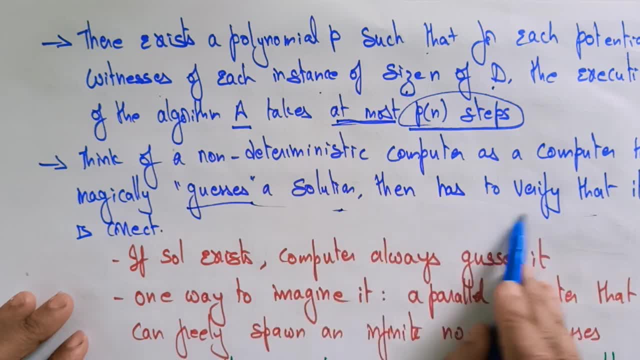 That magically guesses a solution, That has to verify that it is correct. Just think that It is that non-deterministic computer is always magically guessing a solution. Okay, So verifying that it is a correct. If solution exists, computer always gets it. 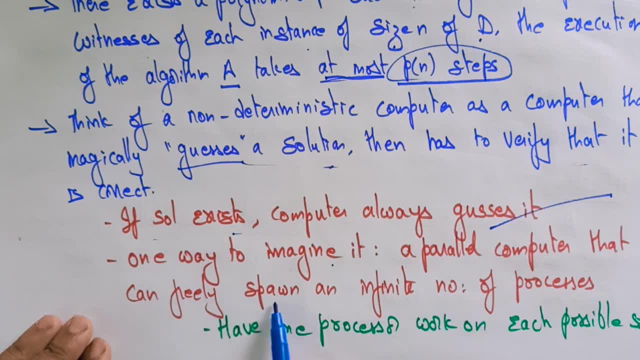 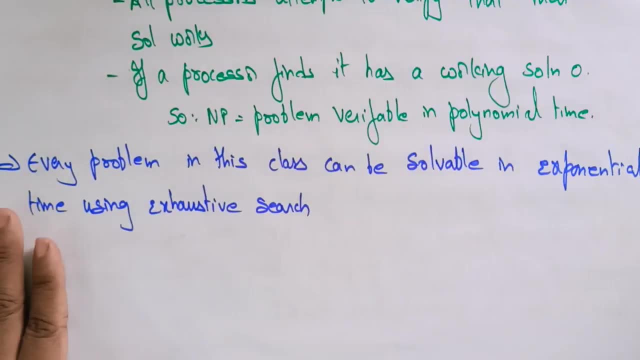 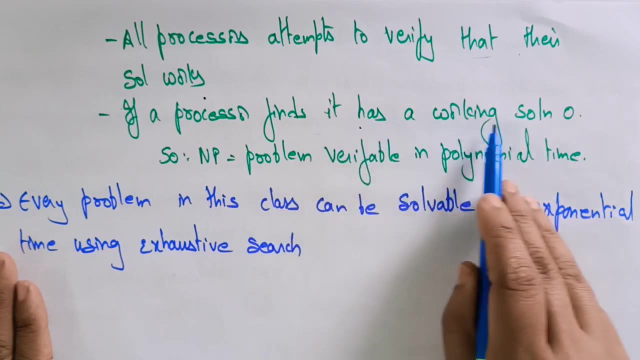 One way to imagine it: A parallel computer that can freely spawn an infinite number of process. That is, It have in one process work on each possible solution, Or all processor attempts to verify that there is a solution work, Or if a processor finds it as a working solution. 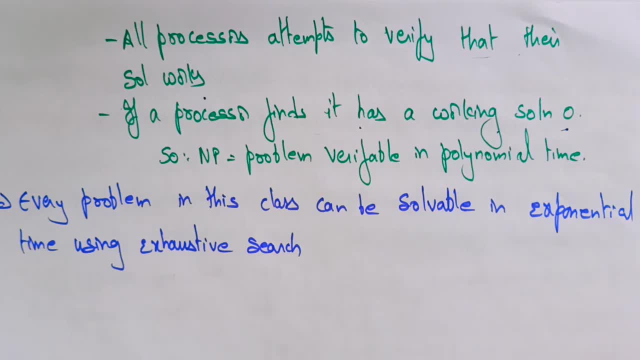 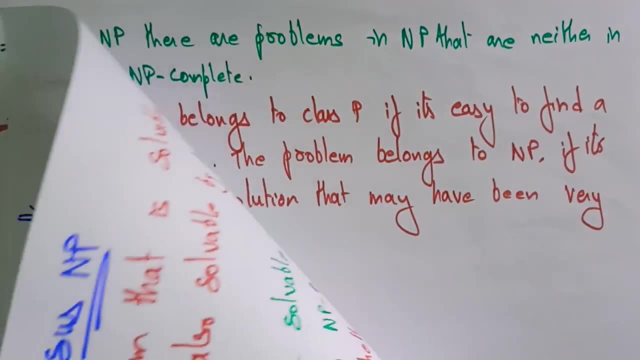 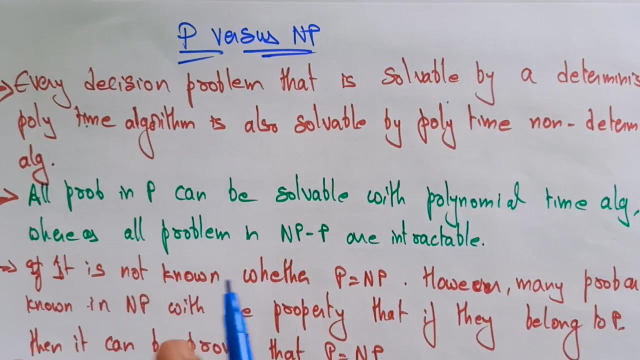 Okay, So the main thing here in the NP class is: every problem in this class can be solvable in exponential time using exhaustive search. Now let me explain you the P versus NP. What is this class? P versus NP- What is the main difference? 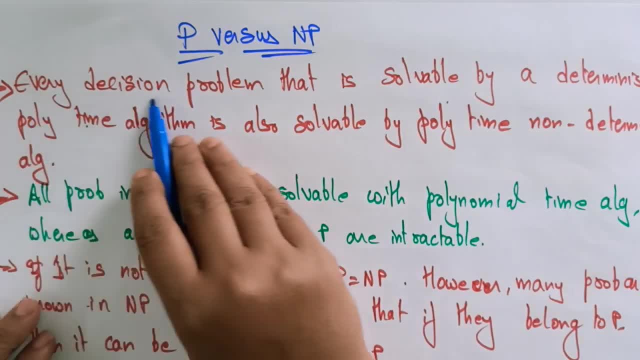 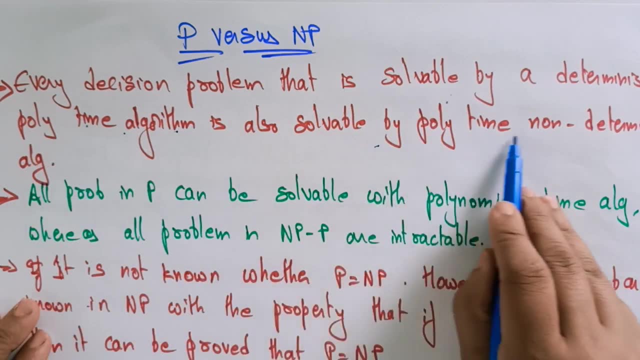 The main difference between the class P and the class NP. Now let us see. Every decision problem that is solvable by a deterministic polynomial time algorithm is also solvable by polynomial time non-deterministic. Okay, Every decision problem, whatever the decision problem you are taking, that is solvable by deterministic polynomial as well as the non-deterministic polynomial. 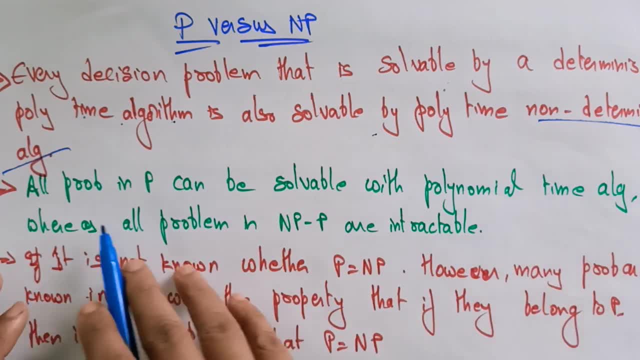 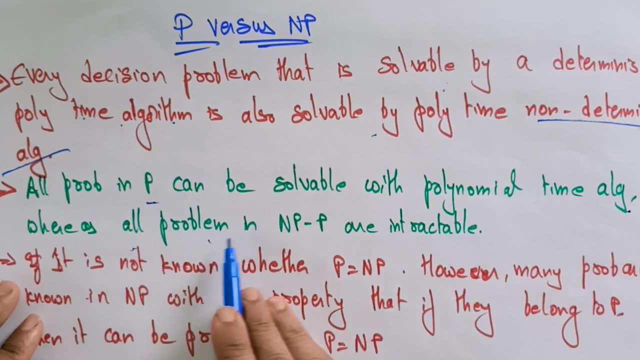 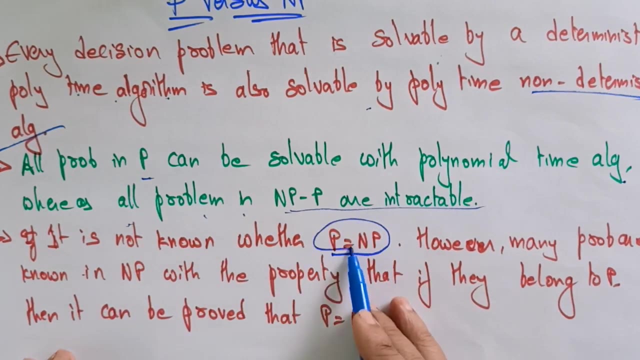 That is the deterministic All. So there is a P and NP. All problems in polynomial P can be solvable with polynomial time algorithm, whereas the problems in NP-P are interactable. It is not known whether the P is equal to NP. 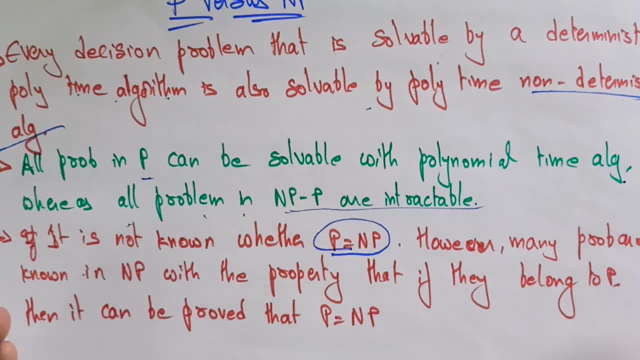 We does not know whether the P always equals to NP or not. However, many problems are known in NP with their property that if they belong to P, then it can be proved that P is equal to NP. So when you can solve, 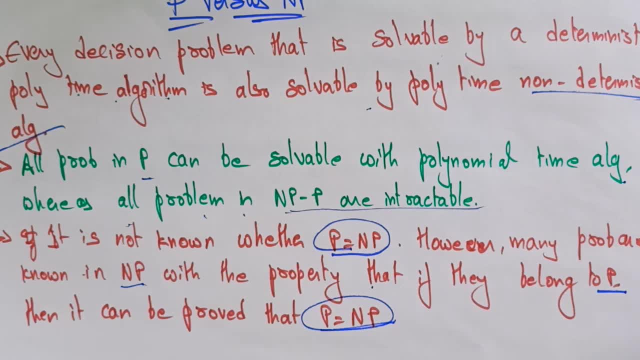 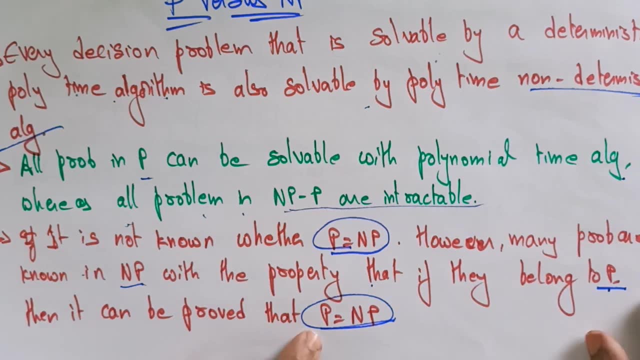 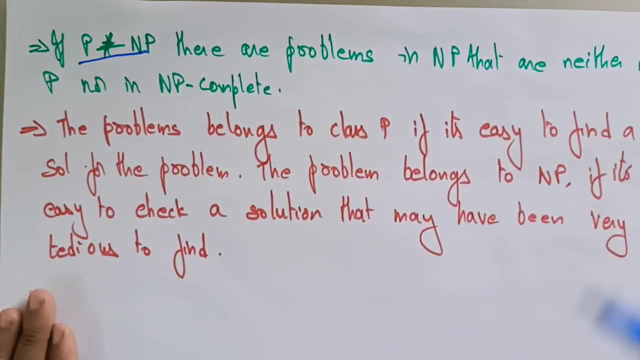 When you can Know that P is equal to NP. So whenever there is a property that, if they belong to polynomial, that can be proved that P is equal to NP. Okay, So if suppose, if let us take- P is not equal to NP? 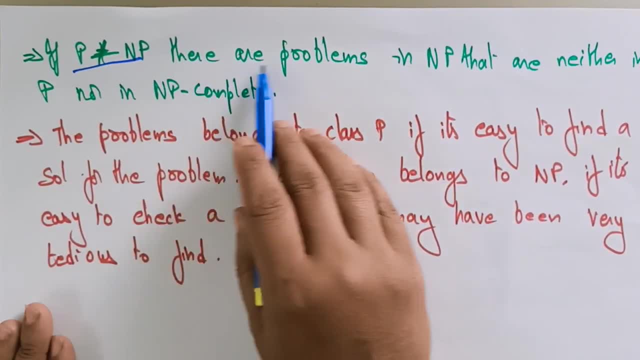 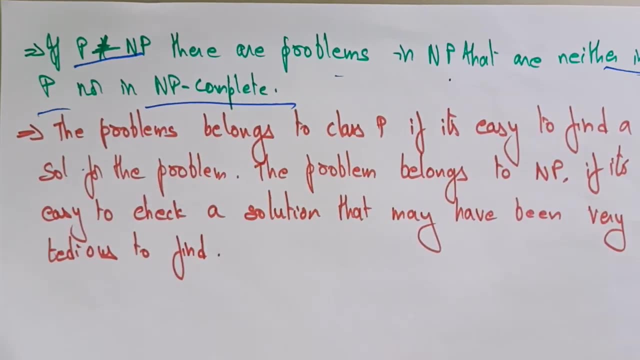 When a P is not equal to NP. If P is not equal to NP, there are problems in NP that are neither in P or nor in NP. So the problems belongs to class P If it is easy to find a solution for the problem. 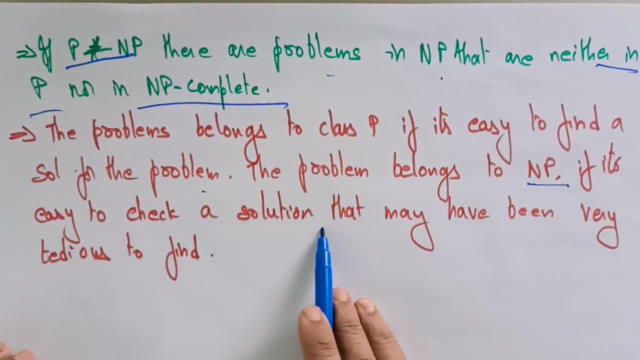 The problems belongs to NP if it is easy to check a solution that may have been very tedious to find. So this is completely theoretical concept. This complexity classes about the P NP. Okay, Completeness of NP. Everything is a theoretical. 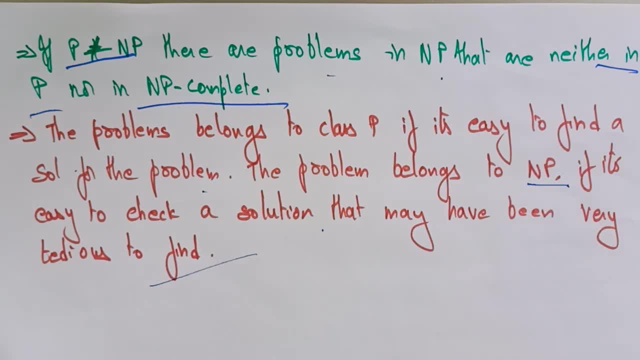 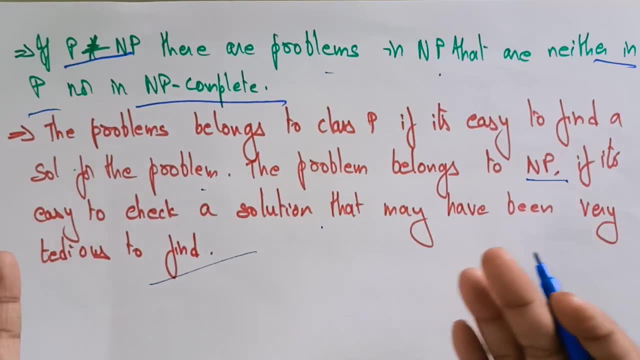 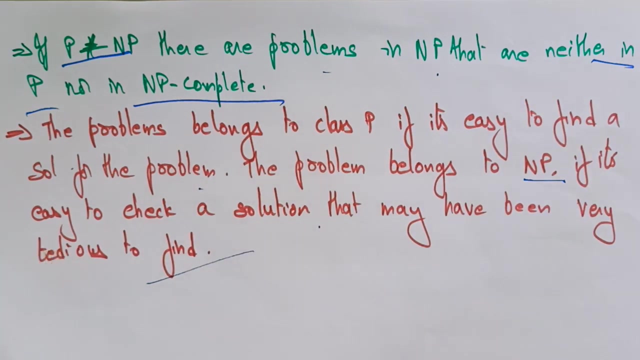 So just go through that theory, Okay, Then you will understand. So here I just read the theory, Okay. So I am not able to give the clear Idea by taking the example. So in the next videos I will try to solve this P class and NP class and explain you with an examples. Thank you.